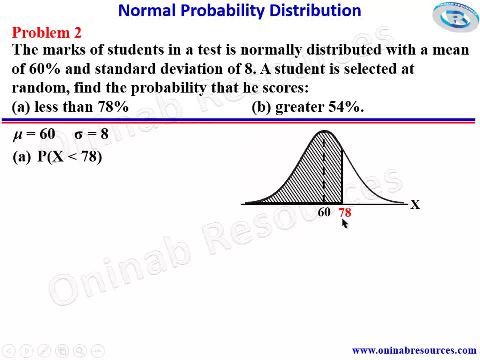 to be having the area of 78. So we are going to be having the area of 78. So we are going to be using the region from the line of 78 to the left, which is the shaded part. So, before we proceed, 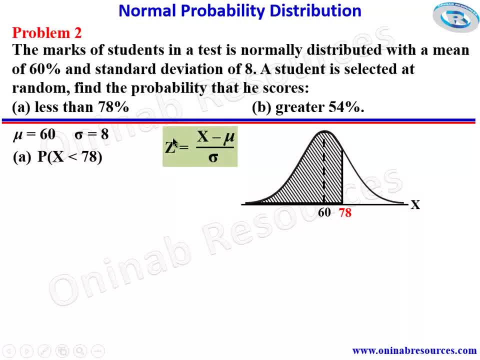 we are going to convert this to z score using this formula, So that our z will be x, which is 78 minus the mean minus 60, then divide by 8.. So, simplifying this, we have 2.25.. So that we now represent the 2.25 in the z. 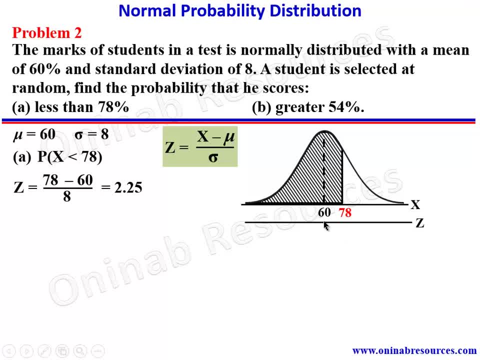 core axis, so representing it on the z axis, remember, the mean is always 0 along the symmetrical axis. then 2.25 here, so that we now have the probability of x less than 78 to be equal to probability of z less than 2.25. to calculate this now, from this 0 to 2.25, we find the probability, let's find the. 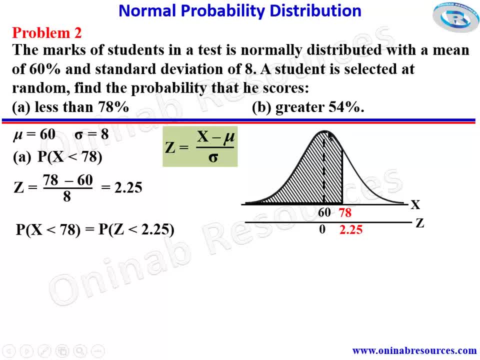 area, from the area under curve table. then this is from this 0 to the end. here is 0.5. so we now say 0.5 plus probability of 0, less than z, less than 2.25. that's from the 0 to 2.25. so we have 0.5 plus. so we look onto the table. so from this table- now we're going to look- 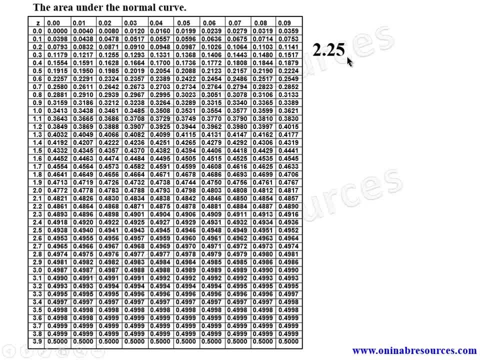 at the area under the normal curve for 2.25. if you see the z score, we are going to split it into 2.2 plus 0.05. our 2.2 is down here under the curve, so we're going to divide by 2.25. 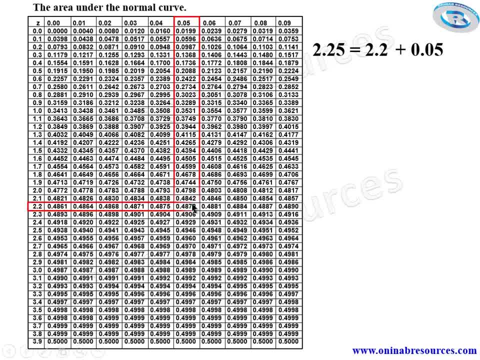 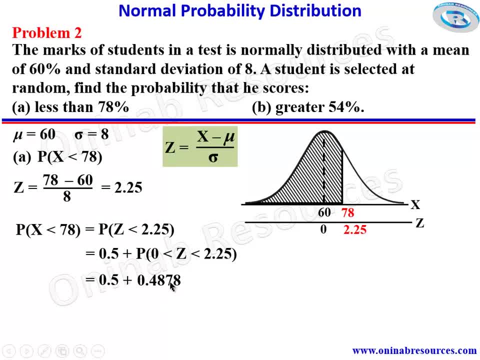 strawberry & submit. and when we look at this table now, 자roll and follow the line here, it multiplied 않는. תחoute is down here under the curve. Motion data tool now has two correspondents. i believe it can analyze this Chinese story again- that 0.05, so that we now have it as 0.4878, to be added to 0.5 and the sum gives 0.9878. 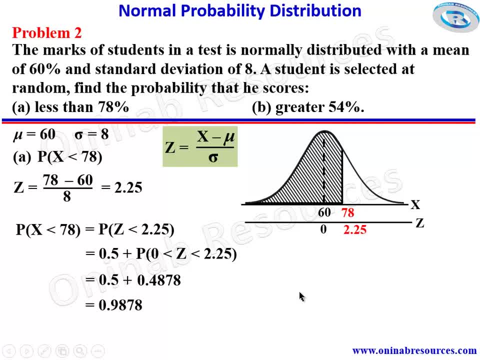 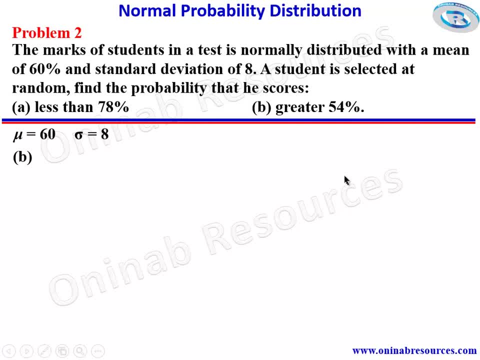 and that's all for 2a. we then go to 2b. for 2b, um, we are to calculate the probability that the student selected at random scores greater than 54. so we look for probability of x greater than 54. this is going to be represented in the normal curve. this is 60. 54 is to the left of the mean. 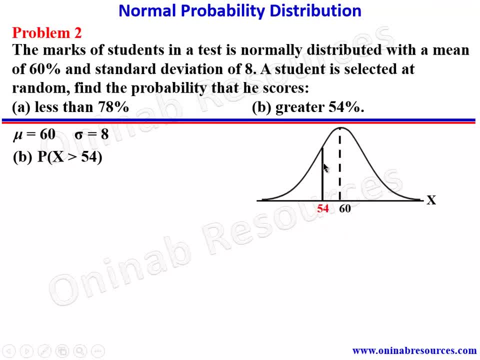 which is 54. here then, since it is greater, it is from this line of 54 to the right that we are looking at, looking for the area which is the shaded part. so what we'll do now is convert the x to z score using this formula, so that z will be equal to 54 minus 60 divided by 8. that gives negative 0.75. 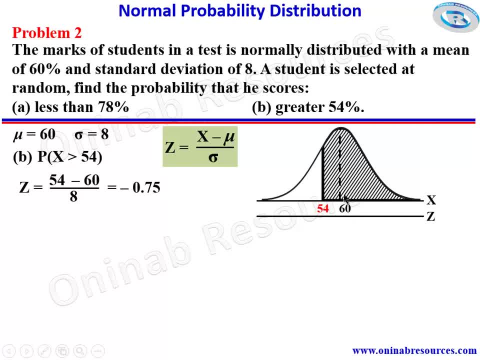 so representing it on the z axis, remember the mean is always 0 along the symmetric axis and here is negative 0.75. remember the area between 0 and negative 0.75 is the same thing as area between the symmetrical line and positive 0.75, so that the probability of x greater than 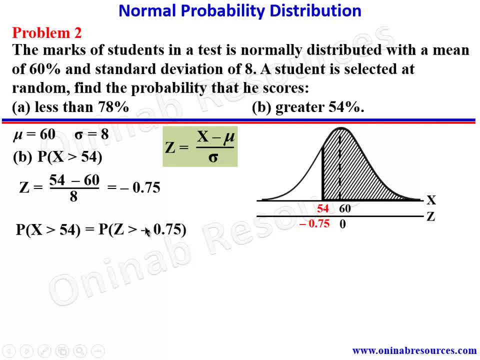 54 will be equal to probability of z greater than negative. 75 from 0 to 0.75 is the same thing as area between the symmetrical line and positive 0.75, so that the probability of x greater than 54 will be. 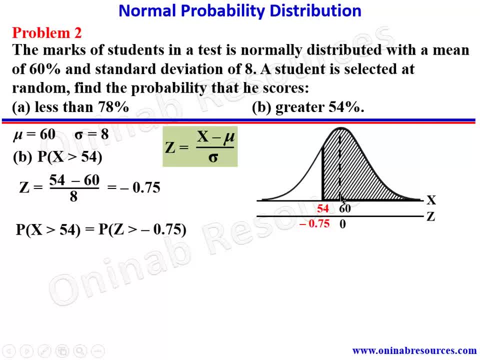 0.75 we find the area, and from zero to the end at the right, the area is 0.5. so we have it as 0.5 plus probability of 0, less than z, less than 0.75. the 0.5 has already been known to be added to this. 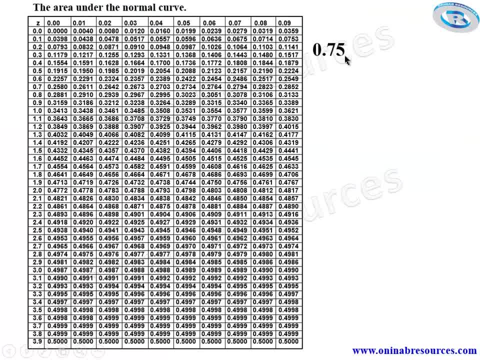 where we check from our table: 0.75, we split it into 0.75, and we have 0.75 plus 0.75 we split it into 0.75, so we have 0.75 plus 0.75, which is 0.75, which is 0.75, plus 0.75, which is 0.75, which is 0.75, which is 0.75. 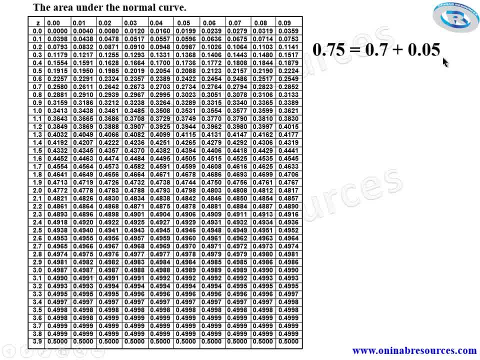 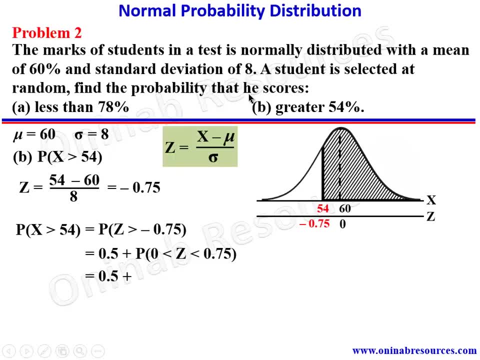 0.7 plus 0.05. we are tracing 0.7 up to 0.05 so that we have our result as 0.2734 to be added to 0.5, adding it 0.7734, representing the probability that the student selected. 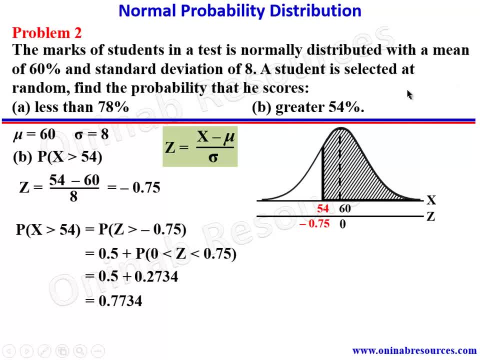 at random scores greater than 54. and that's all for this tutorial. i hope you enjoyed this. thank you for watching. check the description section of this video on our youtube channel to get the link to the first problem and other problems on normal probability distribution and other probability distribution. until we come your way again, goodbye. 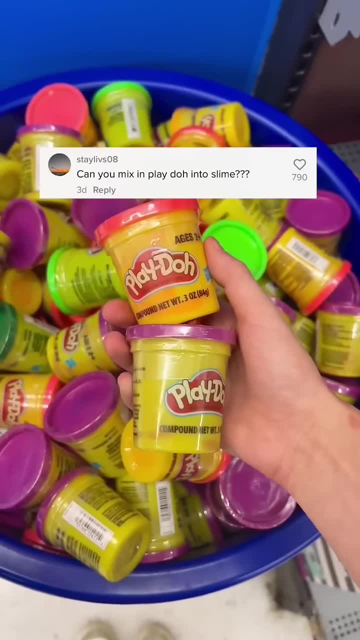 I used to love play with play-doh when I was a little kid. I feel like it was the one thing that got me introduced into slime. I remember when I first played with slime I was really happy that it didn't have the residue that play-doh had, because I hated that, but I really 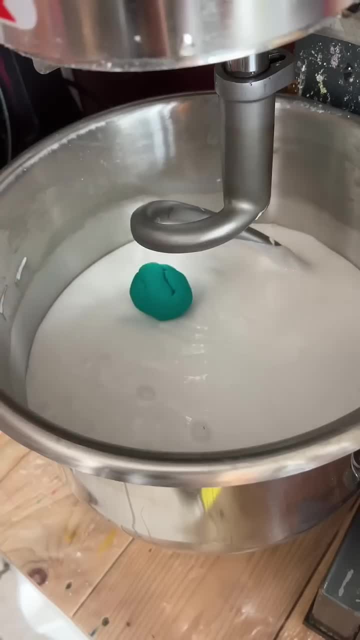 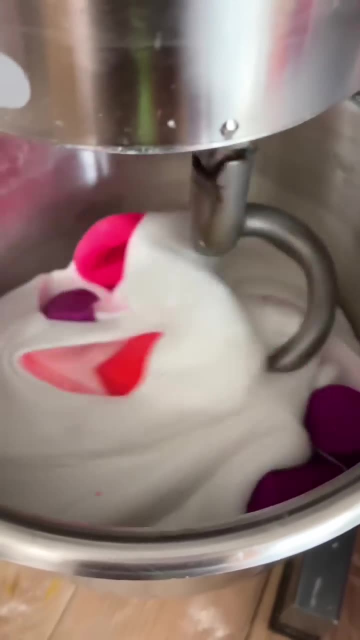 love the texture. If you guys don't know already, play-doh is a kid's toy. It has a really thick and doughy consistency, so mixing with our slime was super exciting. I didn't know what was going to happen. As you can see, I bought a ton of them and I put them all in the mixer. the white glue- 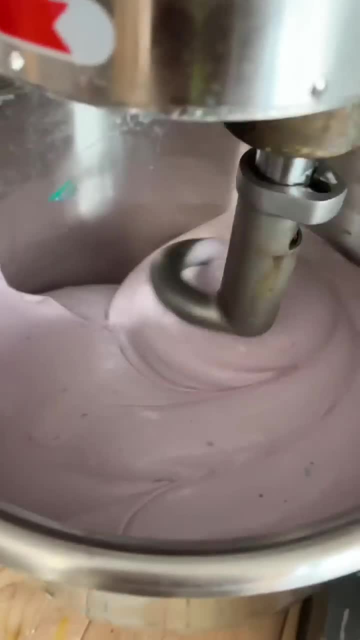 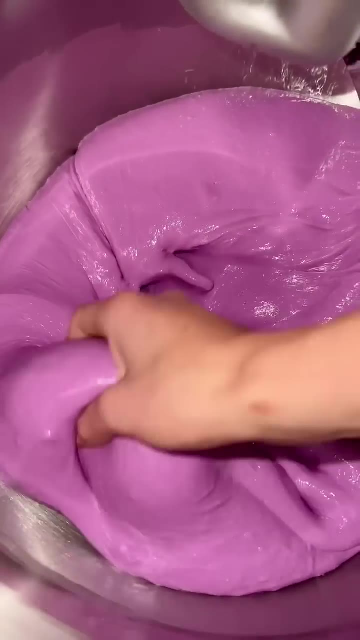 slime and started mixing. I checked in the middle of making this slime. It turns out that the play-doh had actually melted down my slime back into glue. It was so sticky. After adding a lot, a lot, a lot of activator, here is a slime that I managed to make. So that's what happens when you mix play-doh. and slime, You get parakeet dough.